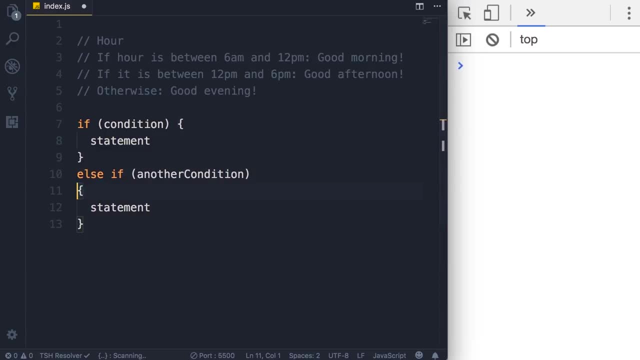 the first curly brace on the same line, not here. that's kind of ugly in JavaScript, so take that into account. now back to our if and else. we could have yet another condition like this, yet another condition: we can have as many conditions as we want, there is no limitation. and once again, here we can. 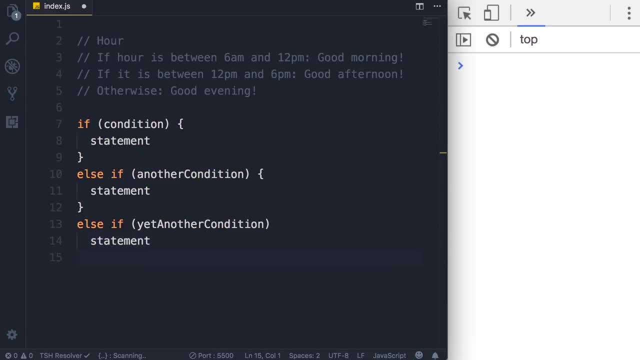 have one or more statements. now, optionally, if none of these conditions are defined, we can put the first curly brace on the same line and here we have multiple terms. conditions evaluate to true. we can use else to execute one or more other statements. so this is the basic structure. now we want to get this logic and map it into the structure. it's very easy. so 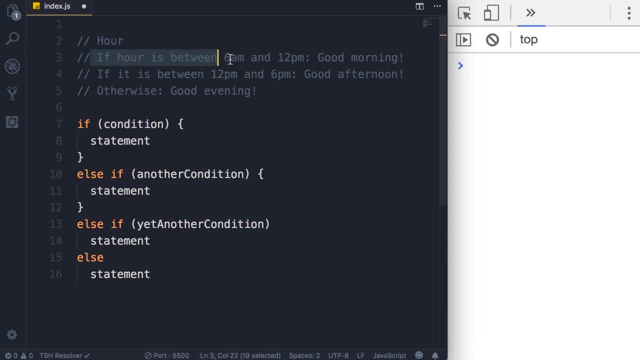 let's start with our first condition. if our is between 6 am and 12 pm, so that's the condition, and the statement we want to execute is: good morning, okay, so I'm gonna declare a variable here hour and set it to 10. now, in a real world application, we want to read the current hour. 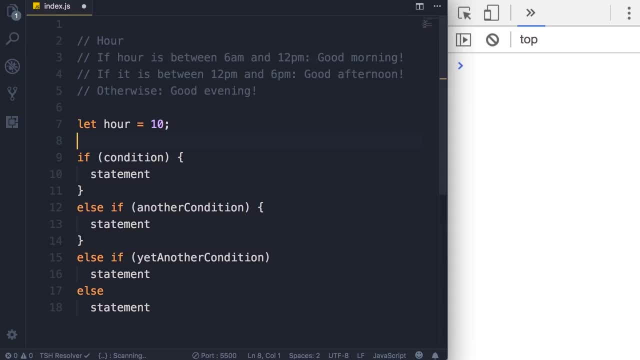 for now, let's not worry about getting the current time and just hard code this number here: 10, okay, so we want to compare the value of our with these two numbers. now, for simplicity, let's go with 24 hour time format, so we want to see if a 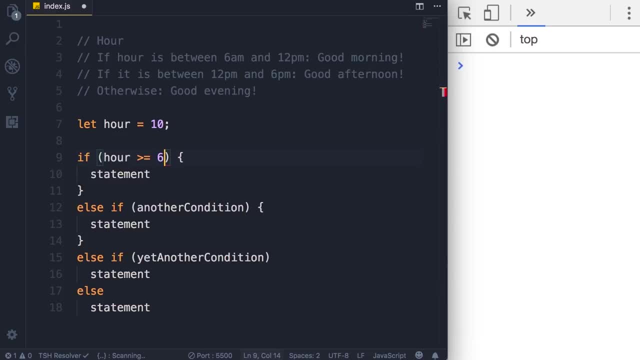 hour is greater than or equal to six and hour is less than 12. you learn this in the last section, right? so here we're using these comparison operators, we have two expressions- here's the first one, here's the second one- and we're applying the logical and in between them. so if both these 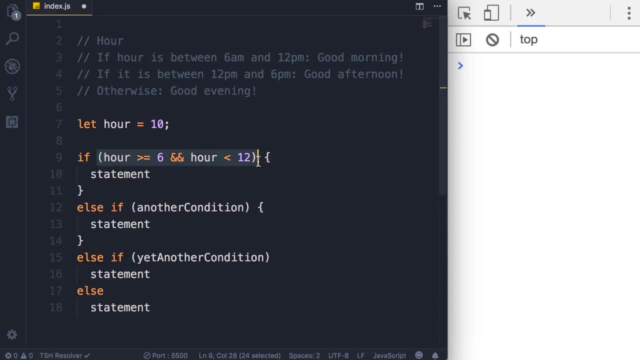 expressions evaluate to true, then the result of this expression will also be true. now let's add the statement we want to display: good morning. and of course, we need to terminate this statement with a semicolon. now here's my suggestion for you. if you want to master javascript, pause the video. 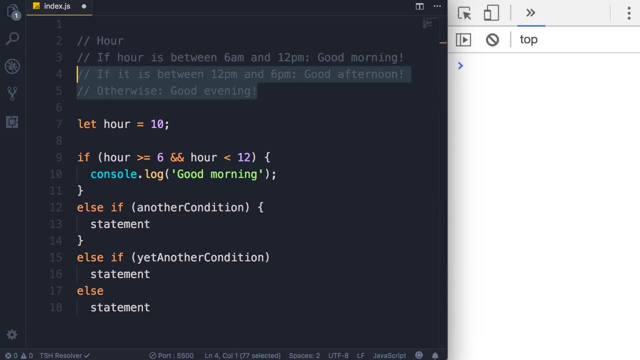 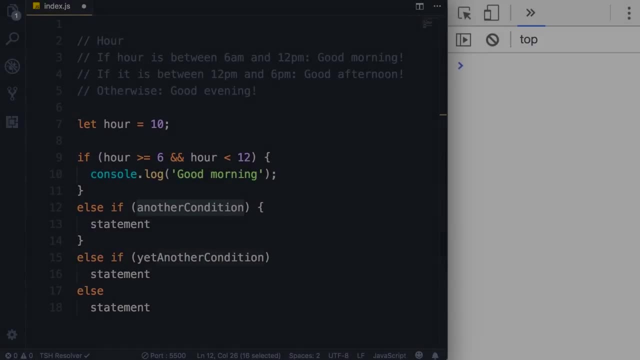 now and continue implementing this logic using if and else. then come back, continue watching and see my solution. all right, let's continue. here's the second condition. we want to check to see if our end result is true or if it's not. we want to check to see if our end result is true or if it's not. 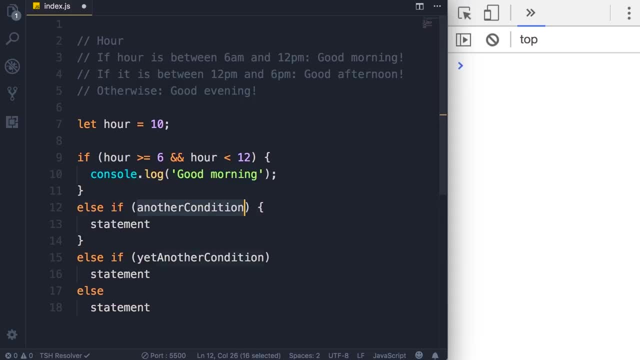 is between 12 and 18, so very easy. if hour is greater than or equal to 12 and it's less than 18, you want to display good afternoon, so consolelog: good afternoon. now in this example we don't need this other il's f, because otherwise we want to display good evening, so let's delete this. 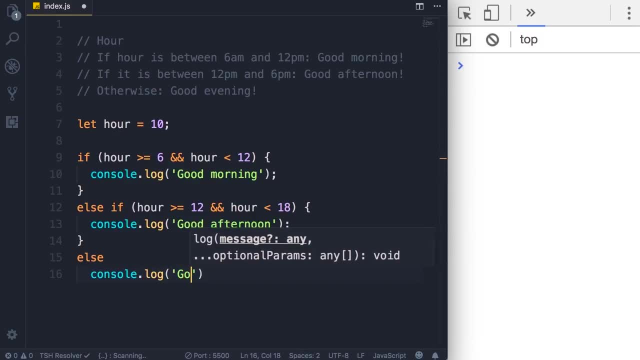 otherwise we do a console dot log of good evening. now, in this example, because we're dealing with a single statement, these curly braces are getting in the way and creating noise in the code, so it's better to get rid of them and simplify the code. here's another pair. okay, that's better. let's save the. 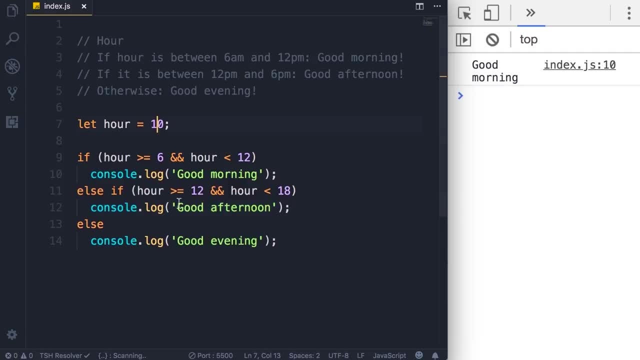 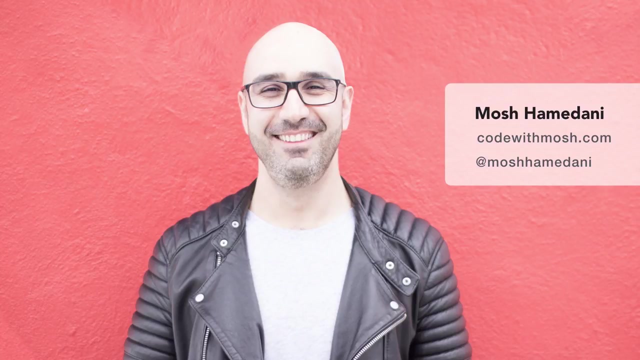 changes. we get good morning here. if i change the hour to 13, we get good afternoon, and if i change this to 20, we get good evening. so this is all about if and else. in the next lecture you're going to learn about switch and case. hi guys, thank you for watching my javascript tutorial, this tutorial. 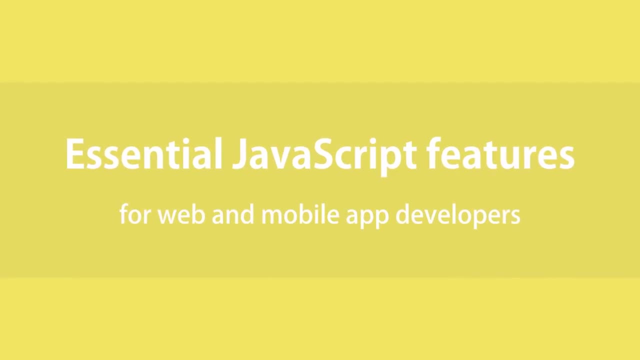 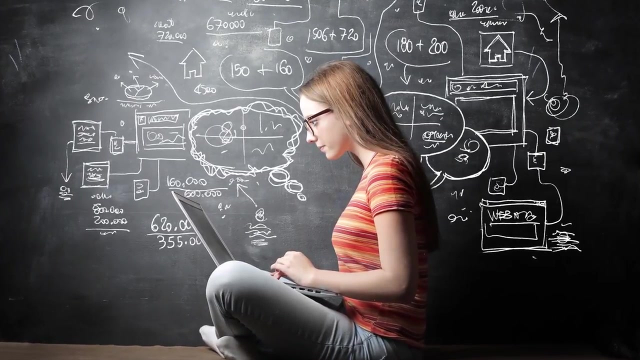 is part of my javascript course, where you will learn all the essential javascript features that every web and mobile application developer must know. if you're an absolute beginner or have some experience in javascript and are looking for a fun and interesting way to use javascript, you can download the javascript learning guide to learn how to use it and how to use javascript in a 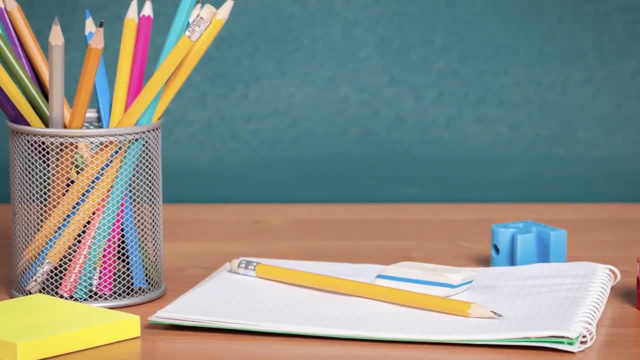 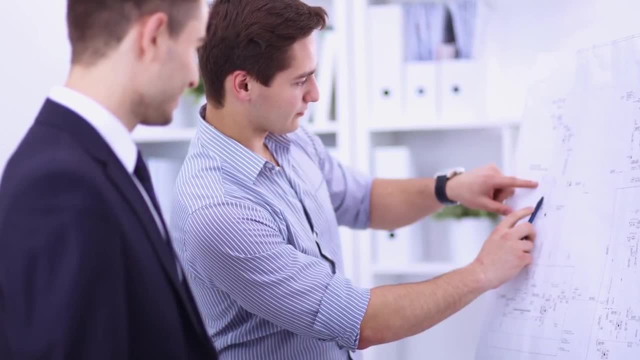 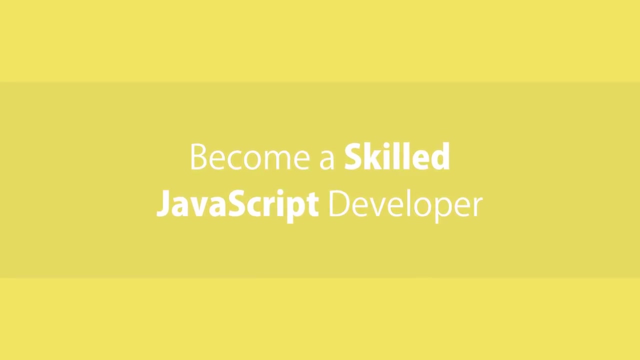 more in-depth course that teaches you the fundamentals of javascript. this course is for you. this course is also packed with tons of exercises that help you master what you learned in the course. in fact, many of these exercises are questions that come up in technical programming interviews. so if you're pursuing a job as a front-end or a back-end developer, or if you simply 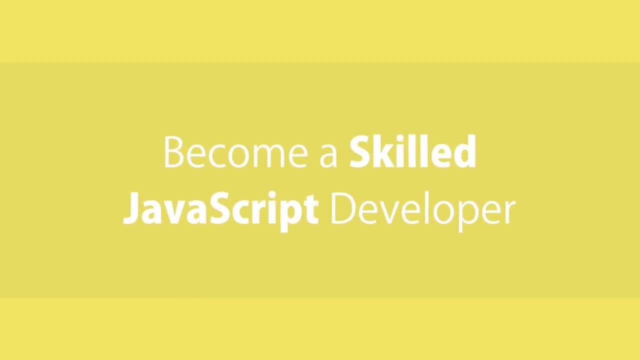 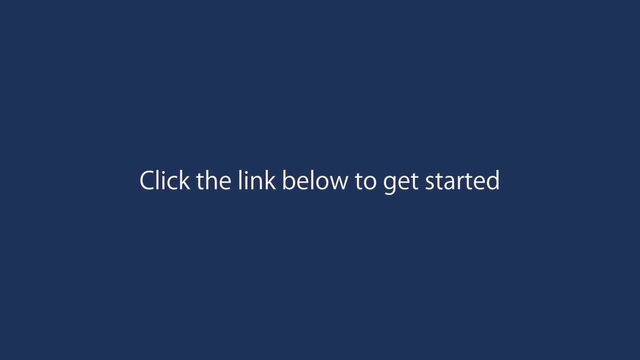 want to have a more in-depth understanding of javascript. i highly encourage you to enroll in the course. for a limited time, you can get this course with a discount for $100.000.. using the link in the video description, Click the link to find out more about the course and enroll.